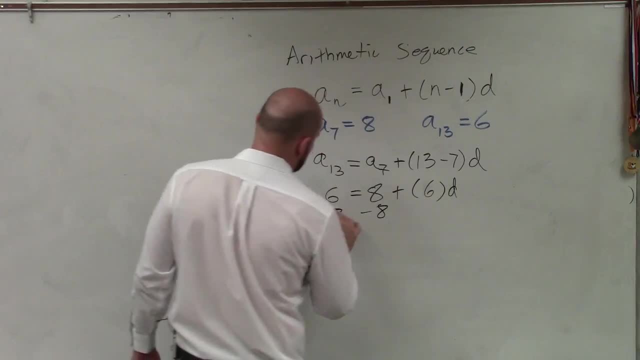 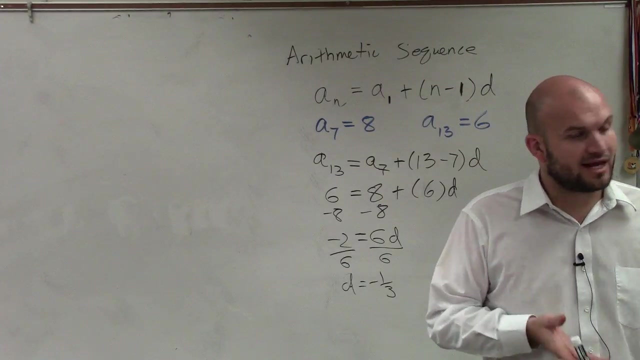 Now I go ahead and solve for d, Subtract 8, subtract 8, negative. 2 equals 6d. Divide by 6, divide by 6.. d equals 6d. d equals a negative 1 third. So now the difference between each and every one of those values is going to be negative 1 third. 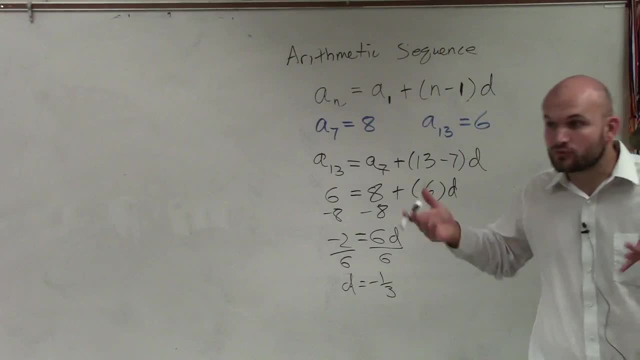 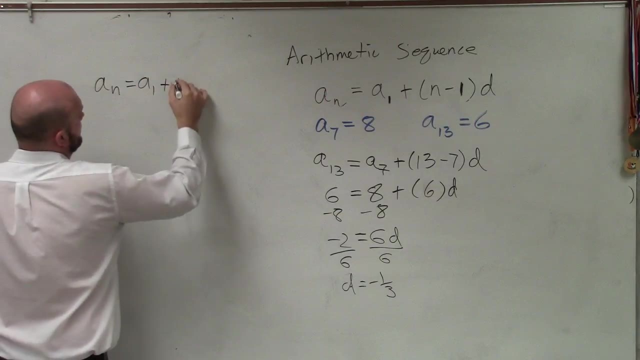 Now again, I still don't know a of 1, right To find this rule. I need to figure out what a of 1 is, So I'm going to go back to the formula. Now again, we can use either one of these: 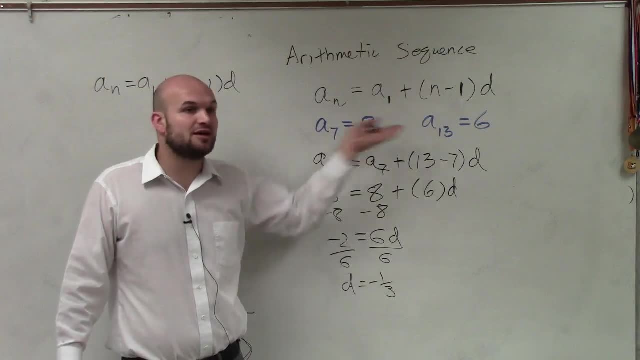 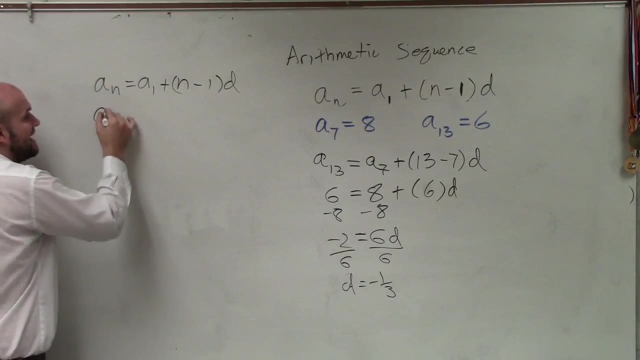 So therefore, I'll ask Dakota: which value would you like to use 7.. Okay, So I need to solve for ace of 1, correct? So I'll say: ace of 7 is the value I'm going to use. equals ace of 1, plus 7 is my n. 7 minus 1,. 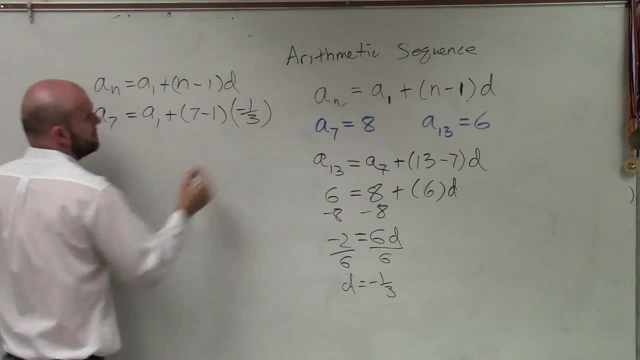 times my difference now, which is a negative 1 third. And now I know the value of ace of 7, right Ace of 7 is going to be 8, equals ace of 1, plus 6 times negative 1 third. 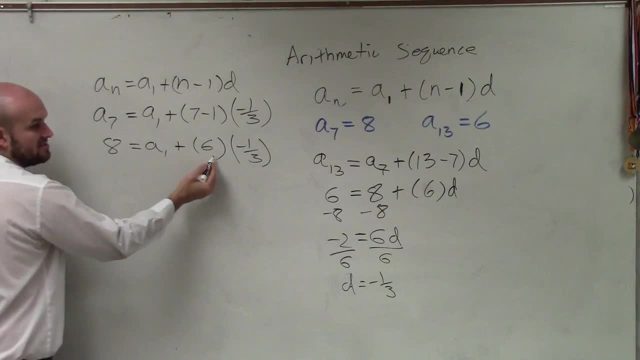 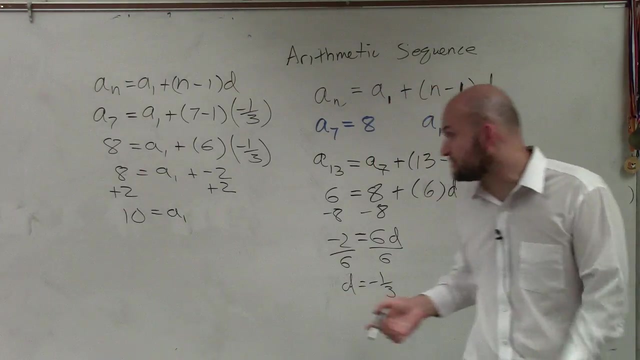 Can I now solve for ace of 1?? Yes, That becomes a negative 2.. 10 equals ace of 1.. So now, if I'm asking you, what is this rule? You guys can see there's a couple steps with this. 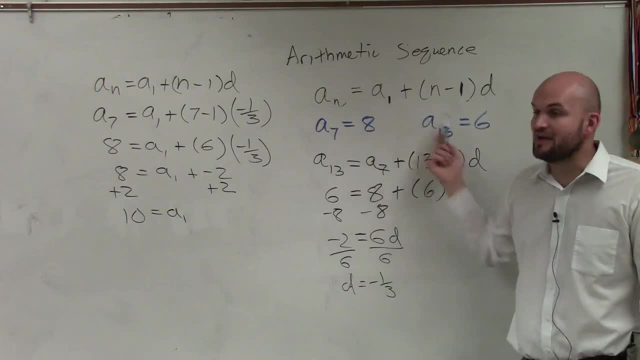 You can solve for ace You know. first you have to figure out the difference. So use the values you're provided to find the difference. Once you know the difference, use ace of 1.. You can use either of these values. 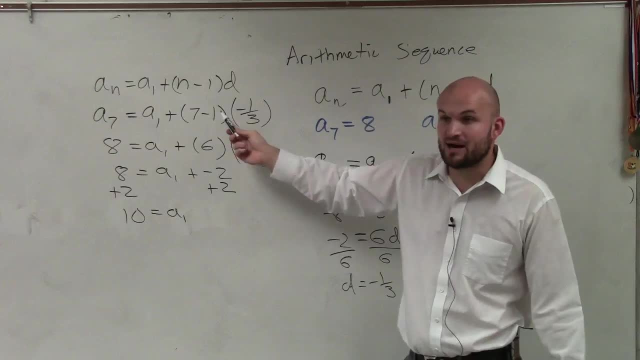 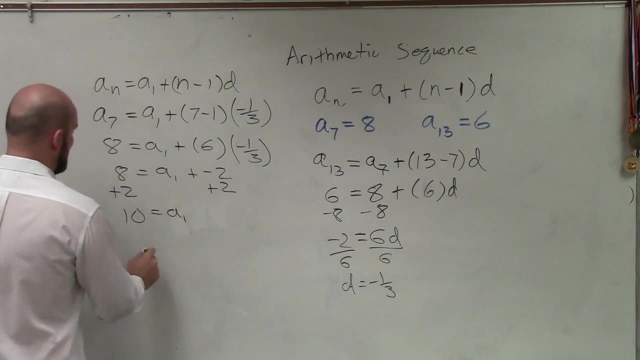 If I were to use ace of 13 and would have done 13 minus 1, right, it would have been the exact same thing. I would have got the exact same answer. okay, McKenzie, But now I know ace of 1, so I go back to my formula. 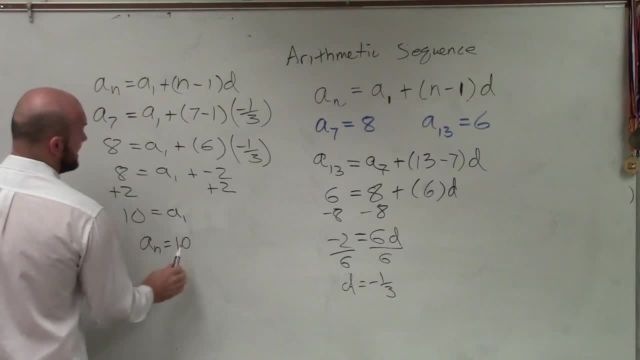 and I say: ace of n equals 10 plus 10 minus 1, times negative 1 third. So ace of n equals 10 plus 9 times. oh sorry, that's what am I doing. So ace of n equals ace of 1 plus n minus 1 times d.